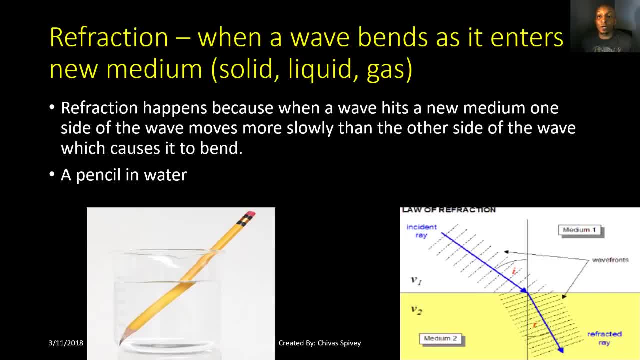 at our next wave behavior, which is refraction. And this is when a wave bends as it enters a new medium, ie a solid liquid or gas. And refraction happens because, when a wave hits a new medium, one side of the wave moves more slowly than the other side of the wave, which 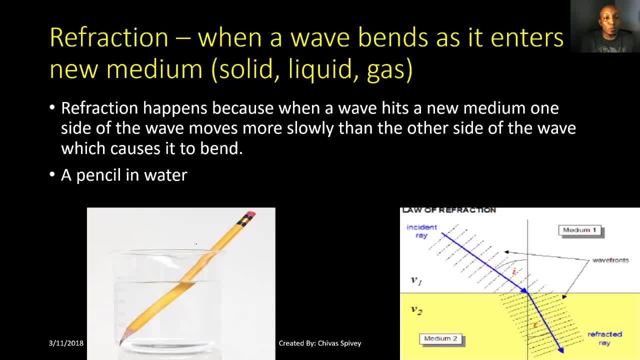 causes it to bend. So if we take a look at this pencil in water that we were in a gas, which was air, and then we moved into a liquid, which is this water right here, And if you notice the pencil looks bent right here, and that's because one part 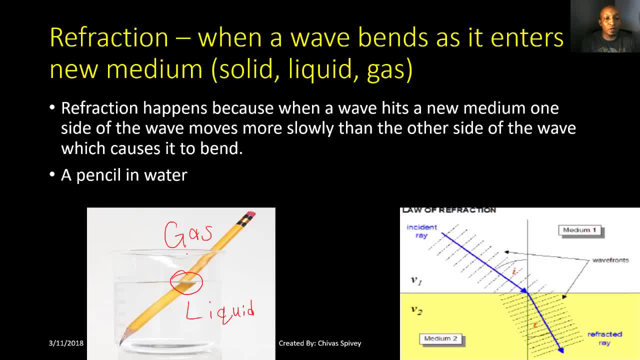 of the wave hits the water before the other part of the wave. So, as the wave goes from medium to medium, or when it goes from a gas to a liquid, one part of the wave hits the liquid before the other part of the wave, which causes this pencil right here to look bent. 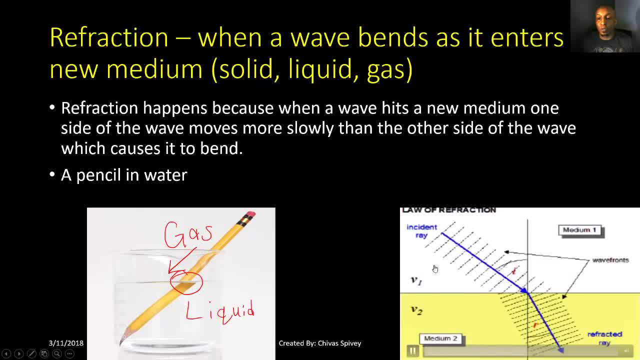 And then, if we take a look at another example, here we are with another wave. so as this wave passes from medium to medium, notice that this side of the wave actually hits this new medium first. So this side of the wave hits it first and then this side of the wave hits it later. 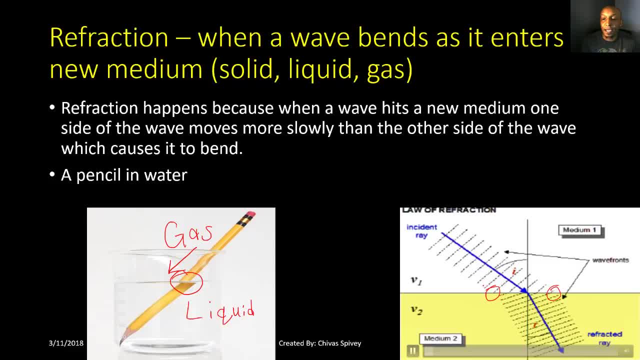 So, since this side hits it first, it causes it to bend on this side and then it causes it to bend on the other. Why does this occur? Because this side of the wave hits first and then this side of the wave hits later, which causes that refraction or that bending behavior. 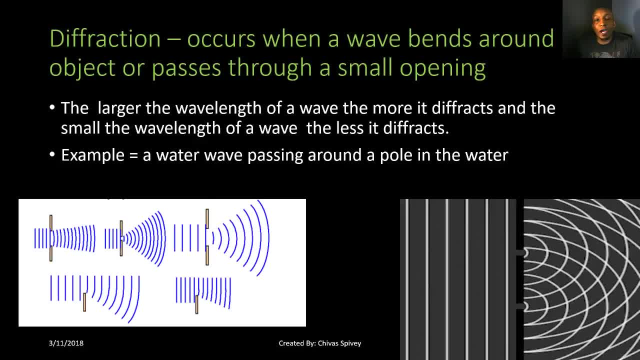 And now let's take a look at diffraction. And diffraction occurs when a wave bends around an object or passes through a small opening, And the larger the wavelength of a wave, the more it diffracts. And the smaller the wavelength of a wave, the less it diffracts. 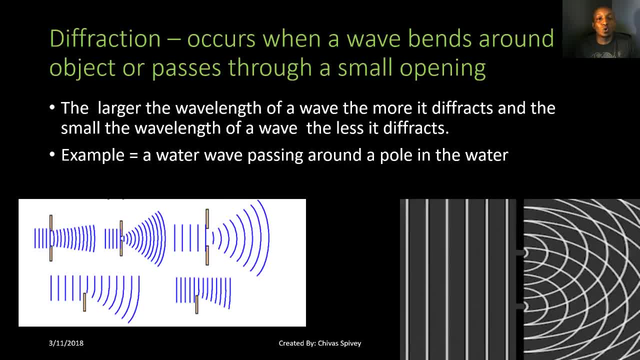 So, for example, a water wave passing around a pole in the water. So let's go ahead and take a look at these different types of diffraction- Notice that this opening right here is large And so a large amount of the water is able to travel through, And look at the angles at which. 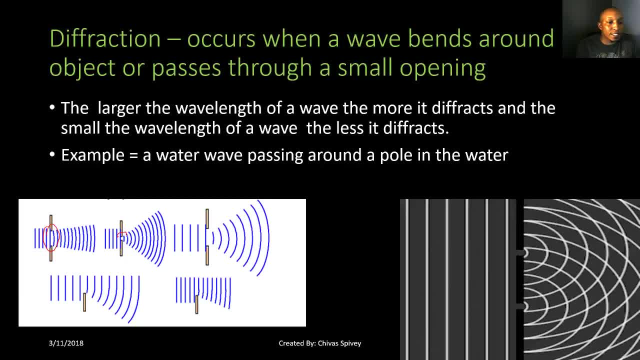 the water comes out. But if you take a look at this example of diffraction, this opening right here is smaller, So most of the water is not able to get through and is actually reflected or bounces off. But a small amount of water that does get through, it actually pushes through. 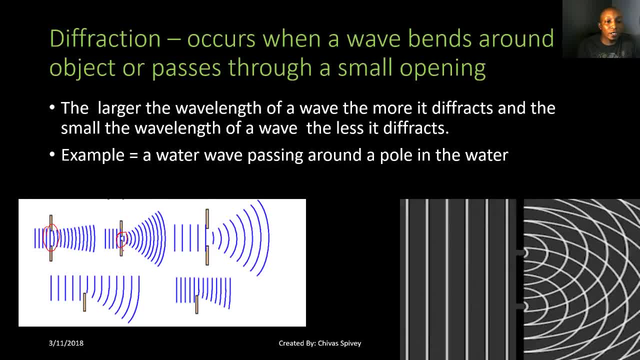 At a certain angle, which causes this angle right here to be larger in this example than from the previous example. Why? Because this angle or this opening is smaller than this opening. Now let's take a look at our next one. So another example. So here's our water wave coming through. 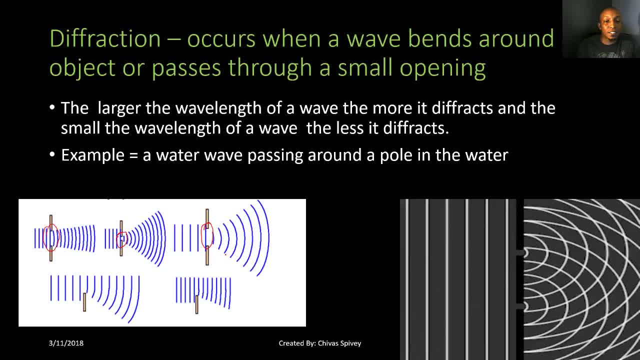 And then, as this water wave tries to bend around this object, look at the angles that it takes as it moves or bends. And then, as it bends, it tries to bend around this object. And so, if we look at our next angle or look at our next diffraction example, notice we have a water wave. 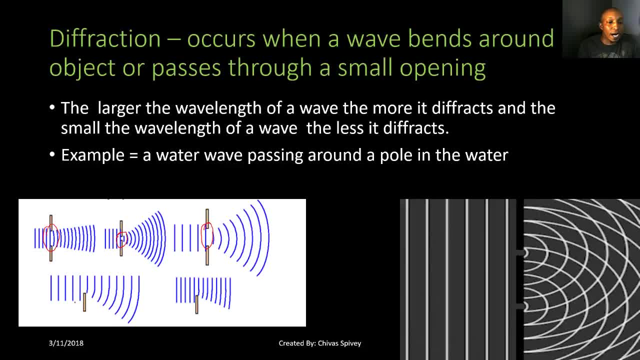 going straight, but then it bends around this object. So some of this water does not make it pass, but the water does make it pass. It bends around this object in this manner. And then, if we look at our last example, it's similar to this example, but we have more. 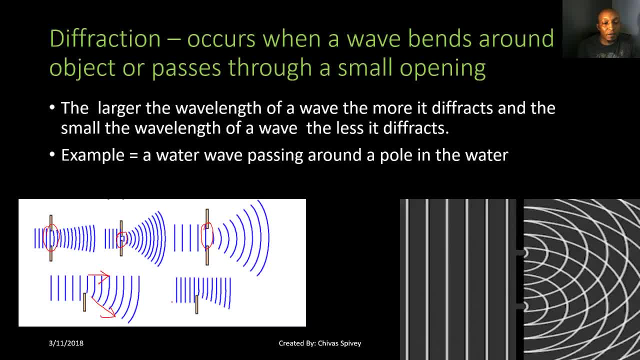 water waves going through. And so if we look at our next angle or look at our next diffraction example, notice we have a water wave going straight, but then it bends around this object in order to move forward. And then let's look at another example. So here are our water waves traveling through. 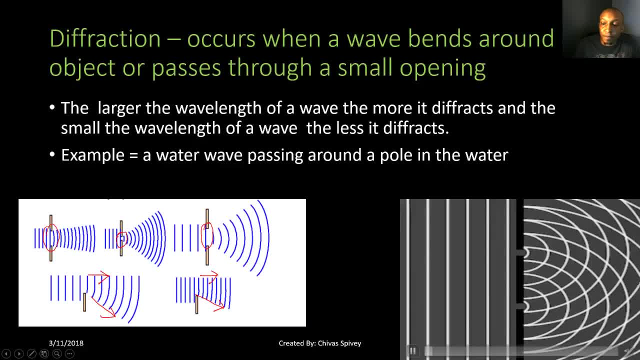 these two small openings And if you notice, these openings are right here and right here And most of the water does not make it through. but the water that does make it through the openings, they travel at different angles as they bend around or bend to get through this. 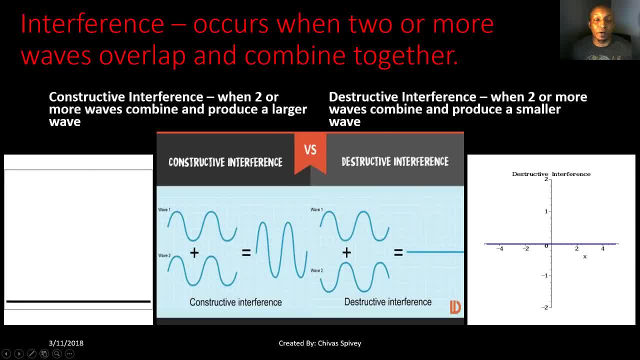 small opening. And now let's move on to wave interference, And this occurs when two or more waves overlap and combine together, And you have two types of interference. You have constructive interference, and this is when two or more waves combine and produce a larger wave, And then you 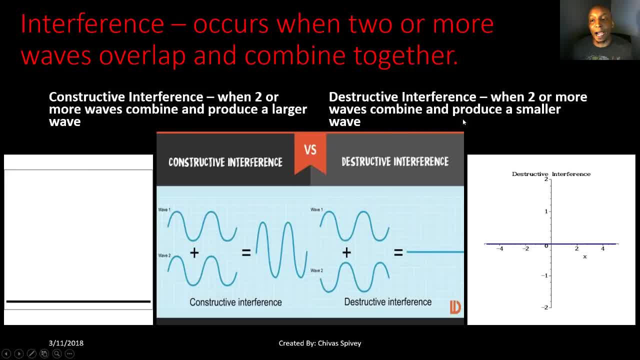 have destructive interference and this is when two or more waves combine and produce a smaller wave. Now, one way I like to think about this is when two or more waves combine and produce a larger wave And I like to relate. it is that constructive interference is that when you got 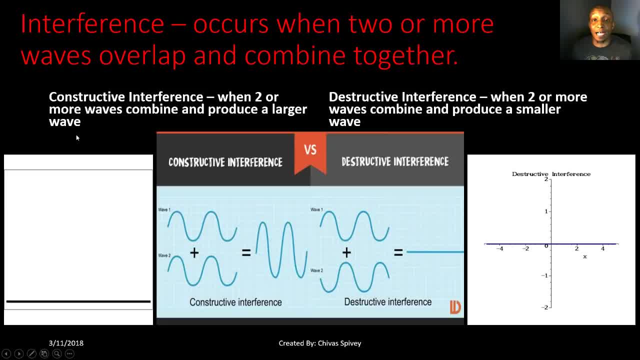 two or more friends that come together and y'all create something positive, something good. that means y'all make a larger wave, something positive or great. But then when you have destructive interference, you got those certain friends that come in your life or those certain 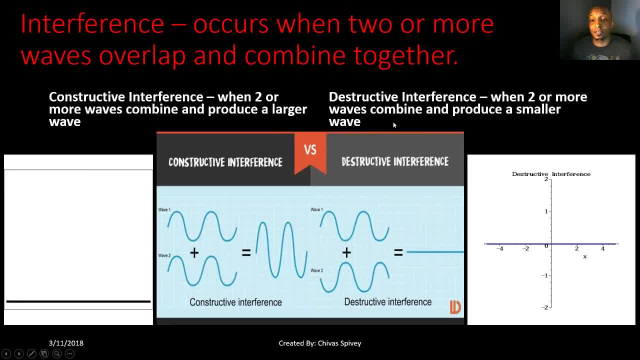 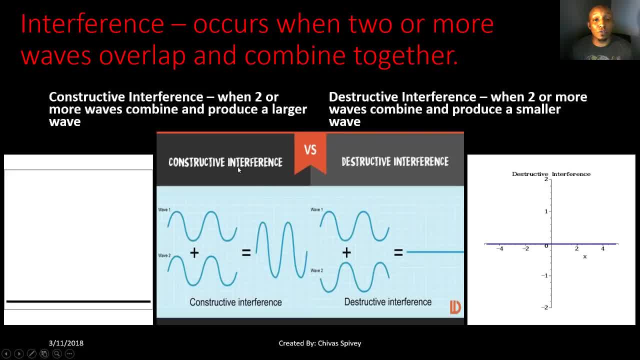 on. But let me go ahead and get into the science of this. So if you look at constructive interference, here's wave one and here's wave two. So here's that wave one, here's wave two, And you notice, when these two waves get together, they create a larger wave. They create a larger. 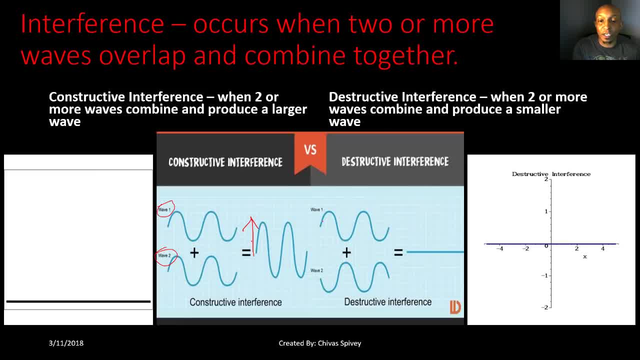 wave. And now let's look at destructive interference. Here's wave one for destructive interference and here's wave two. And then when you combine these two waves together, they create a smaller wave wave. They actually end up canceling each other out. And the reason why this happens- for constructive 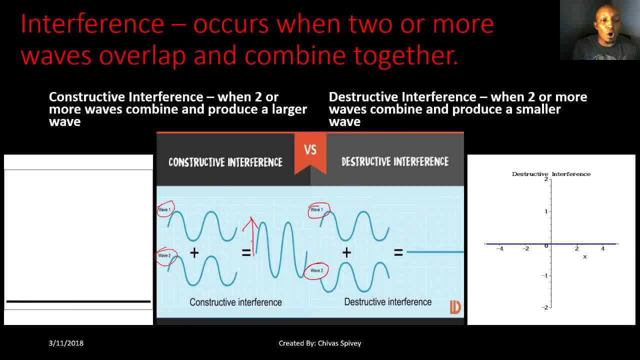 interference. if you notice, both of these waves are traveling on the same wave path, So both of them are moving together in the same wave path. So when you combine those waves together, they create something even greater. So that's what I meant by having good, positive friends in your life. 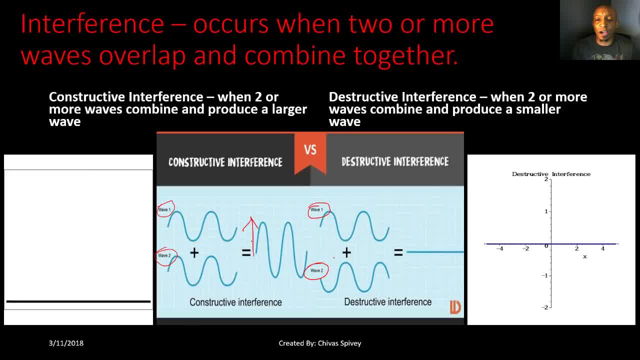 And now, if you notice, if you look at these two waves, these two waves are traveling in opposite directions. When this one's at the crest, this is at the trough. When this is at the trough, this one's at the crest. So when they meet each other, they end up canceling each other out, and 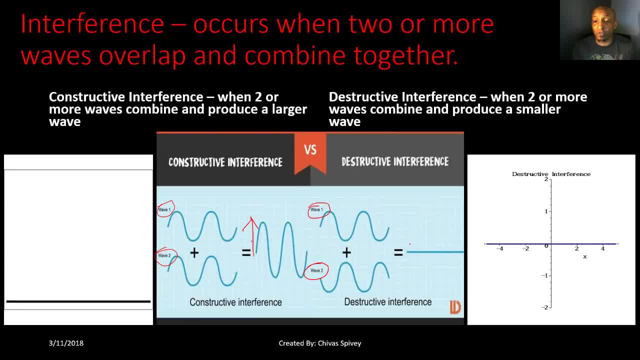 taking away from each other's energy, And this is called destructive interference. These are the type of people that you do not want in your life. So I'll go even further and give an example of this. So here we are with constructive interference. Notice that these two waves 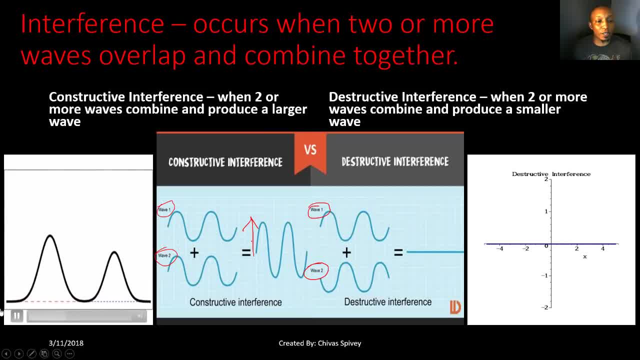 come together and they create something larger. They create a larger wave. So we have something extremely positive going on right here, And here's our example of constructive interference. Now let's look at our example of destructive interference. And if you notice, I got two waves coming from opposite sides, but then, when they get together, 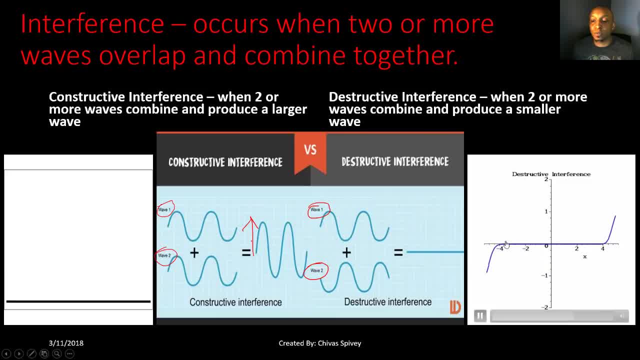 they cancel each other out. So, if you notice, those waves was coming from opposite sides And then, when they came together, they end up canceling each other out. And these are the type of people and individuals or friends that you do not need in your life. You need to. 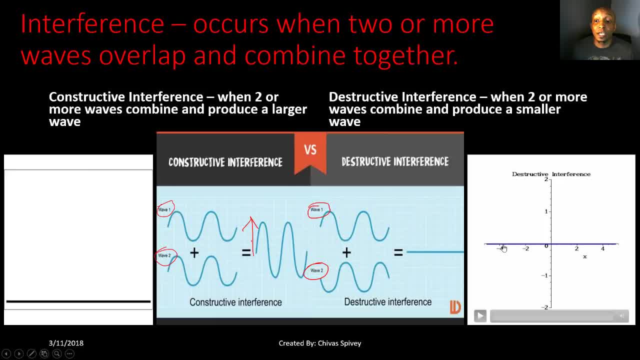 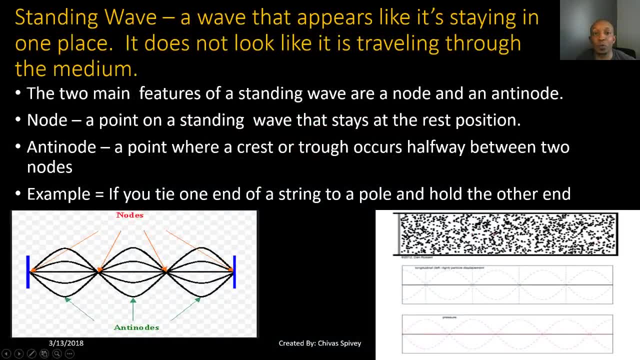 let those people go, because they're going to bring down your energy and cause you to have smaller waves, ie have smaller success in life. And now let's take a look at standing waves. And standing wave is a wave that appears like it's staying in one place. It does not look like. 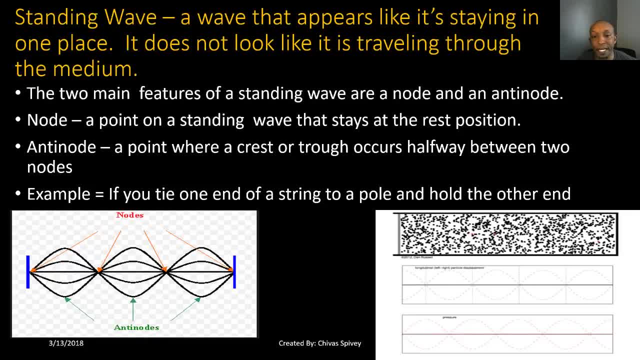 it is traveling through the medium And you have two main features of a standing wave, which are a node and an antinode. And a node is a point on a standing wave that stays at the rest position. So, for example, if you look at this wave on the bottom, 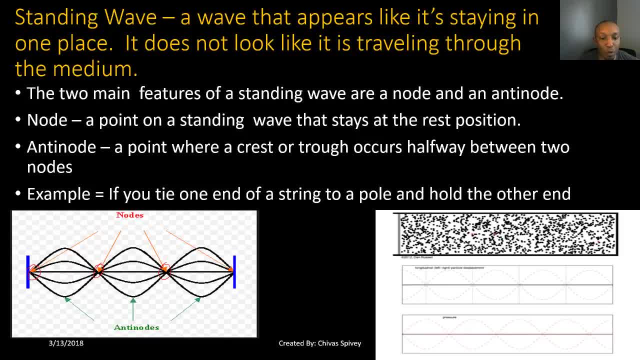 left. we have four nodes on this wave And the way we can tell is because they're at this rest position or at this equilibrium position. And then, if you look, we also have antinodes, And these are a point where a crystal trough occurs halfway between two nodes. So let's take a look. 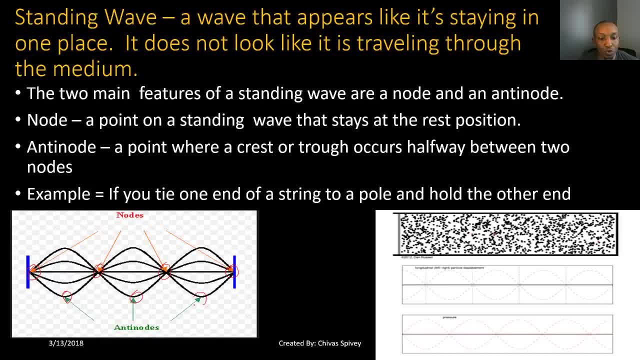 at our antinodes. So we have one, two, three antinodes on this wave. Now, another difference between a node and an antinode is that a node is not carrying any energy And the way we can tell is that it's at the rest position or the equilibrium position An antinode is carrying. 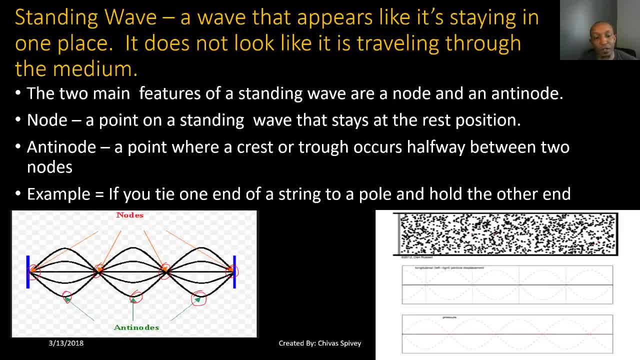 energy. And the way we can tell is because it's moved away from the rest position. So if you look, here's our rest position right here, Here's the antinode. This antinode is carrying energy. And then, if we take another look at a standing wave, notice, if you look at this wave right here. 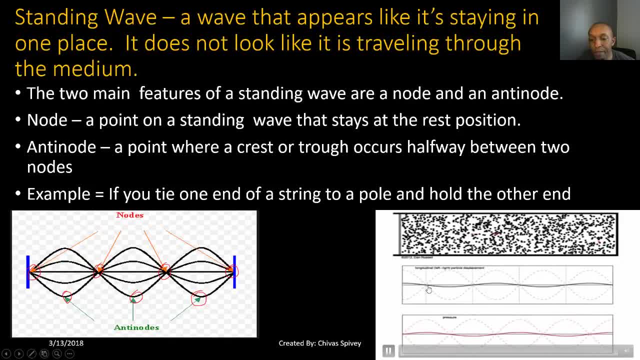 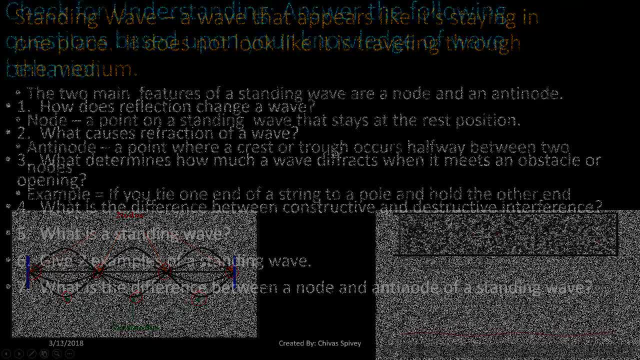 here are nodes right here. They stayed at rest position, And then there are antinodes, And the antinodes moved away from the rest position And they are carrying energy. Now it's time for your check for understanding, And you're going to answer the following questions based upon your 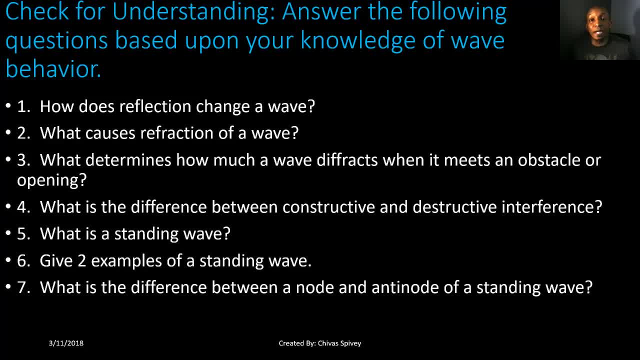 knowledge of wave behavior. You can go ahead and pause the video now as you answer the questions, And I'll make sure to make my way around the room to check on your answers to ensure that you understand the learning for today. Ladies and gentlemen, I'm Colt Spivey, joined by my son. 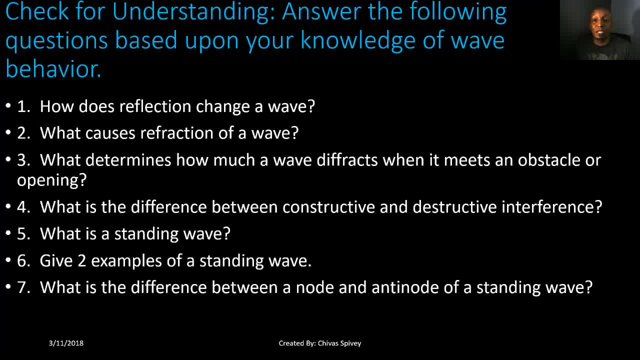 Jordan Spivey, And I hope this wave behavior tutorial was helpful and beneficial. Ladies and gentlemen, make sure that you have a great day And I'll see you in the next video. Bye, Have a wonderful, peaceful, positive, awesome day And remember that you are loved and that. 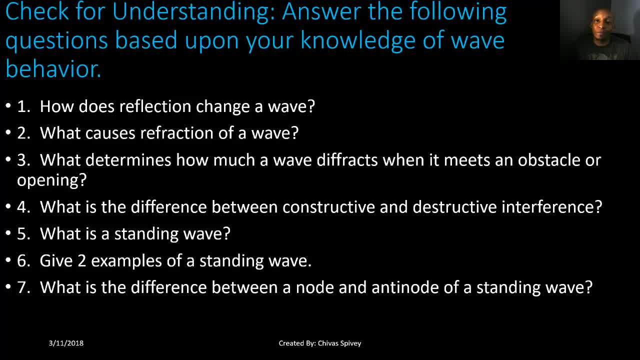 you are cherished and that you are cared for Peace and have a wonderful day.